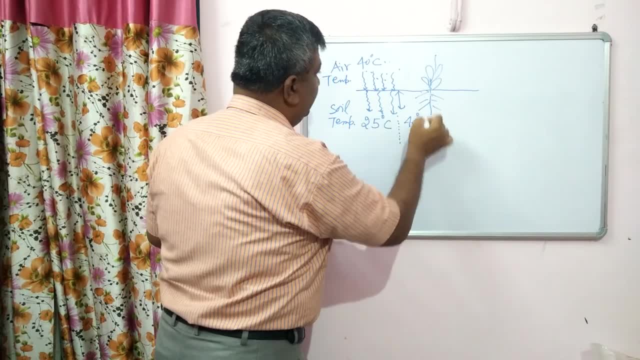 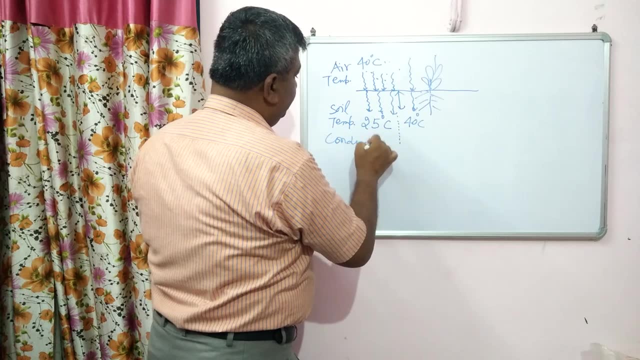 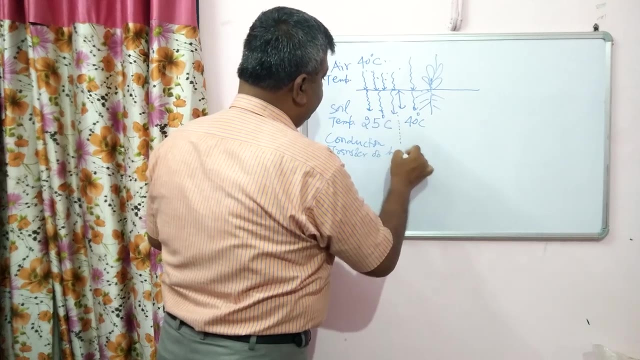 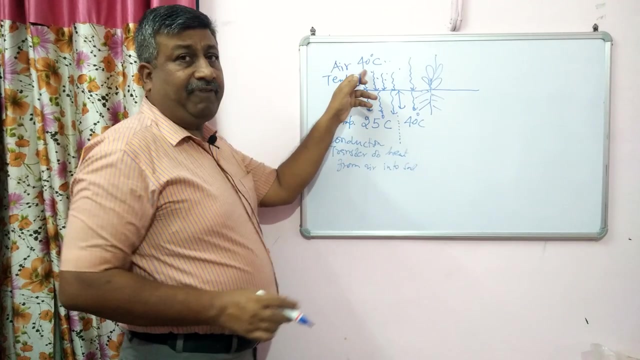 temperature. now this temperature become 40 degree centigrade because of conduction of heat. So here there is a conduction of heat or transfer of heat. We can say transfer of heat From air into soil. Now it is 45 degree centigrade. Suppose heat waves are there. Then the heat. 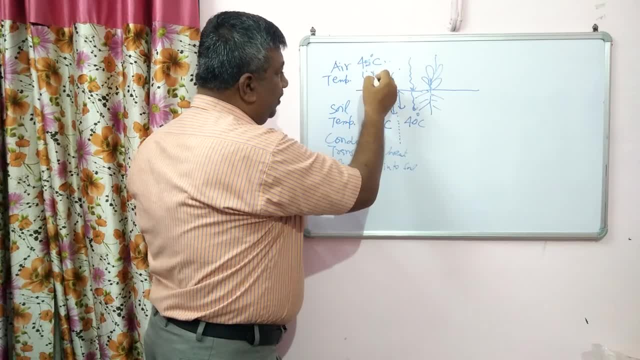 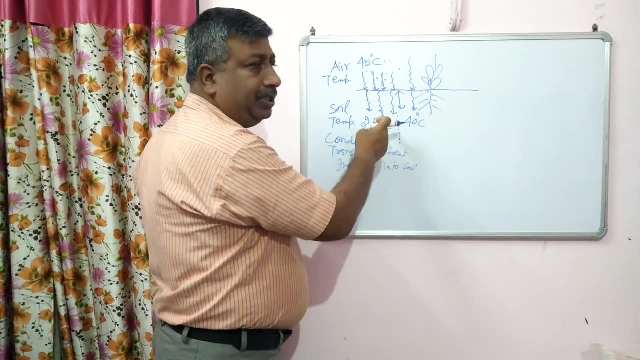 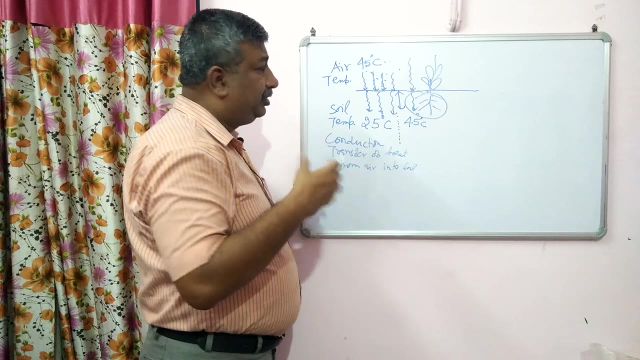 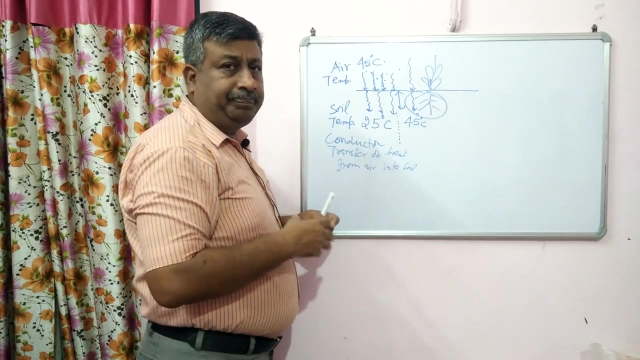 will transfer. Now it is 45 degree centigrade, Then further high temperature on the soil surface, then heat transfer through conduction process into the deeper layer, into the root zone, and temperature become 45 degree centigrade. After the transfer process the temperature of the roots is increased, So temperature is. 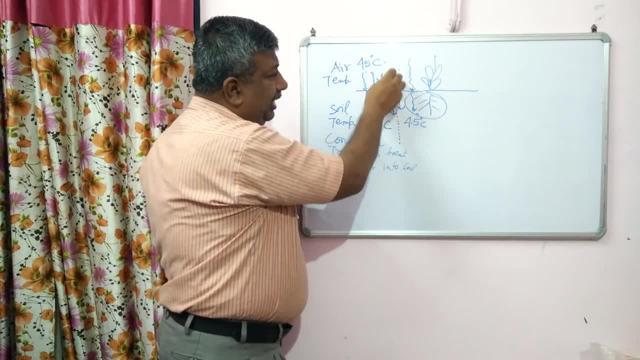 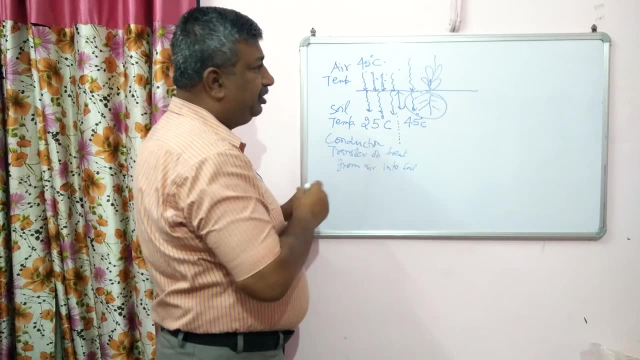 increased. So if temperature is increased in the summer season then the heat will also reaches the soil surface In summer. the heat will get burnt here and here will also get burnt, But the heat will transfer from root to root process through conduction process. 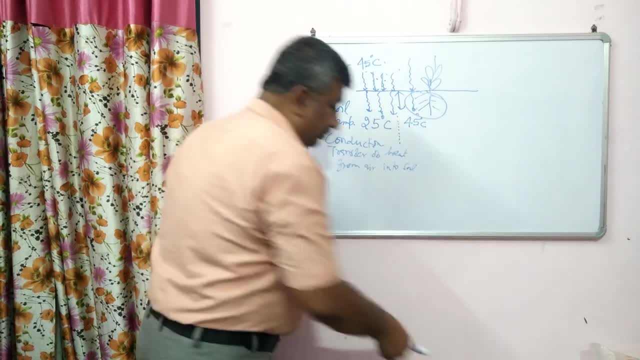 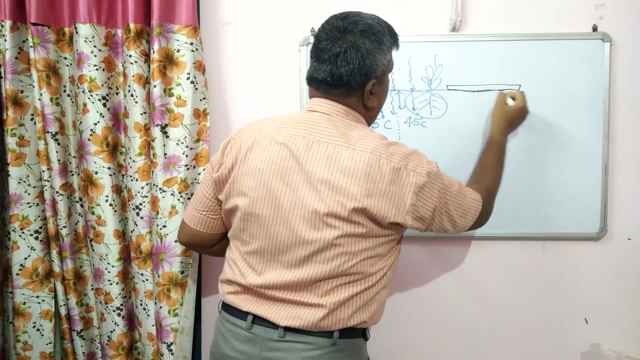 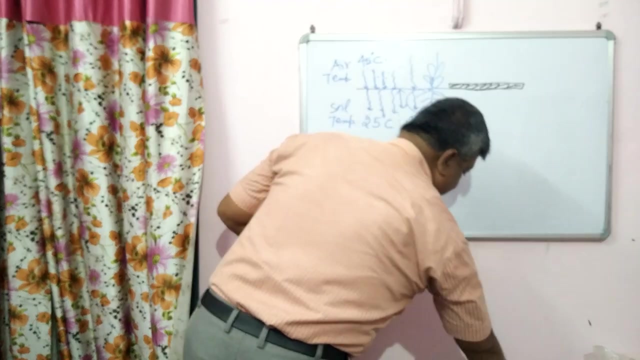 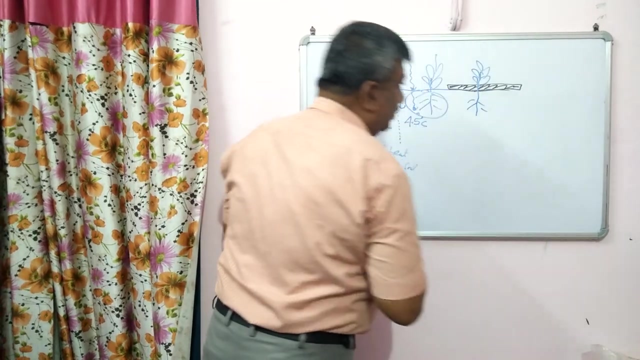 So this is the problem. suppose if we are using organic mulch- now it is organic mulch, crop residue may be crop residue or straw or stover, and this crop residue and the plants are there. plants are there and it is spread over the soil surface and this crop residue. 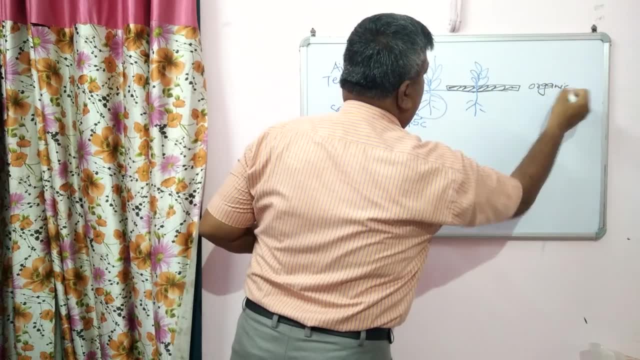 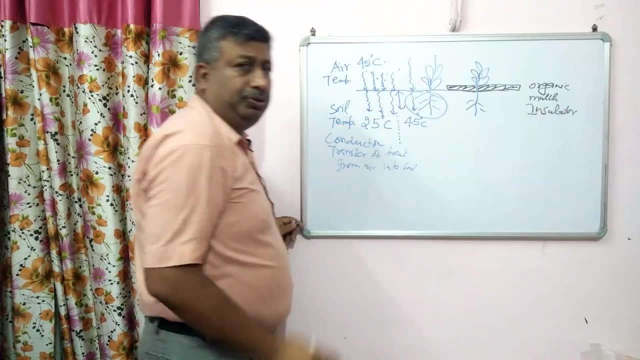 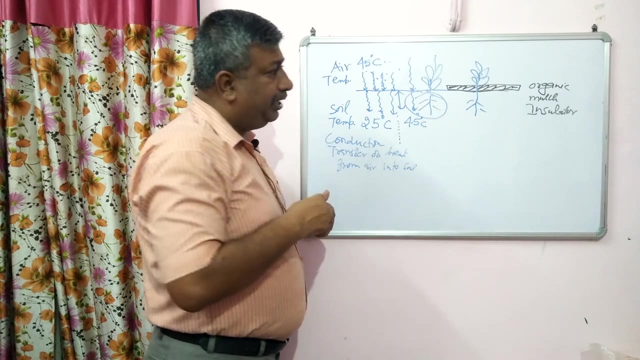 or organic mulch. this is the organic mulch. it act as a insulator. insulator are those substances which do not transmit the heat, so it works like an insulator, and insulator are those which do not allow heat to transfer. so organic mulch may be crop residue very 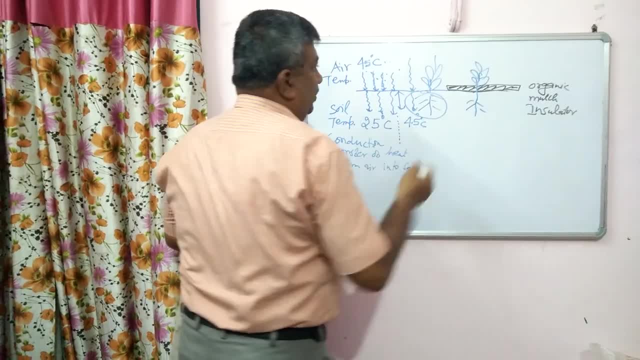 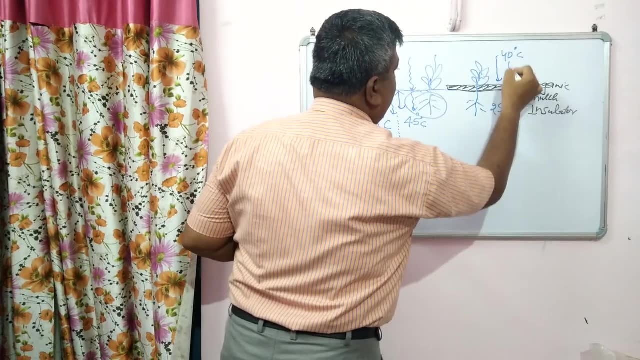 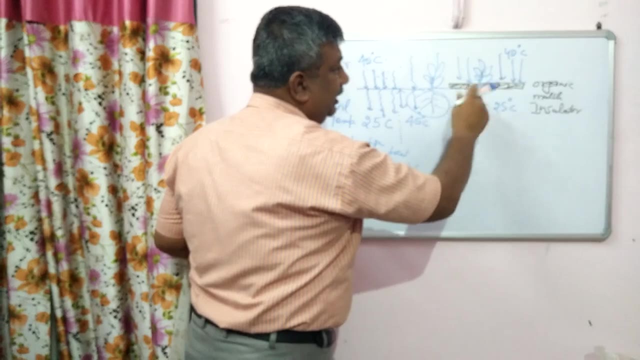 common, or stover or straw. and now suppose temperature is 40 degree centigrade and here temperature initially is 25 degree centigrade. Now the heat is strike on this mulch, but this because this mulch act as a insulator. 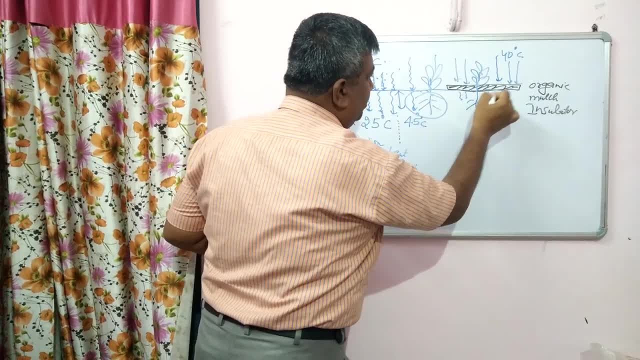 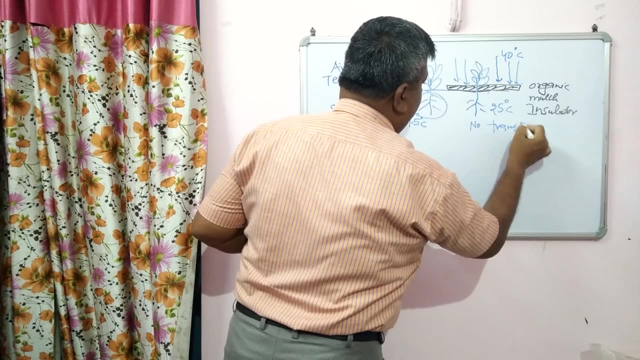 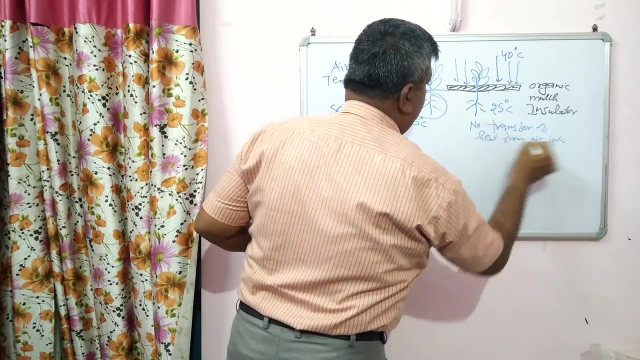 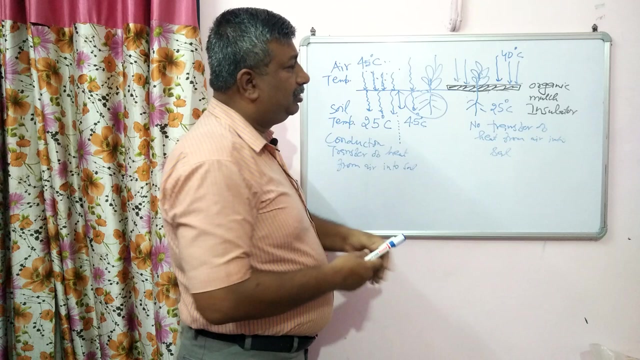 it is not transferred, not transmitted, there is no transmission, no transmission, no transmission or no conduction, or no transfer of heat. no transfer of heat from air into soil because organic mulch are there, And which is the problem? Organic mulch act as a insulator. if we are using organic mulch, then this heat will strike. on the residue or any stover on organic mulch. that mulch works like an insulator. insulator does not conduct heat, so heat will not transfer down and temperature will remain almost 25 degree centigrade. Now air temperature is 40, but here temperature is maintained 25 degree centigrade, suppose. 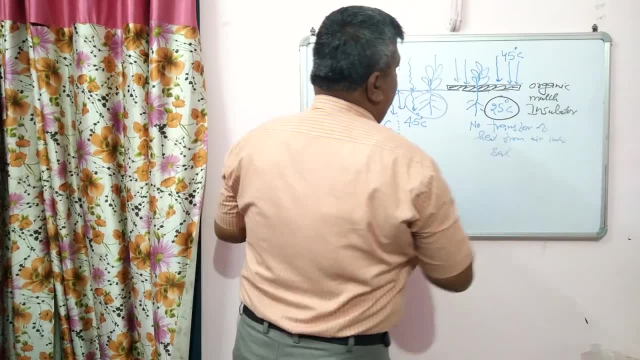 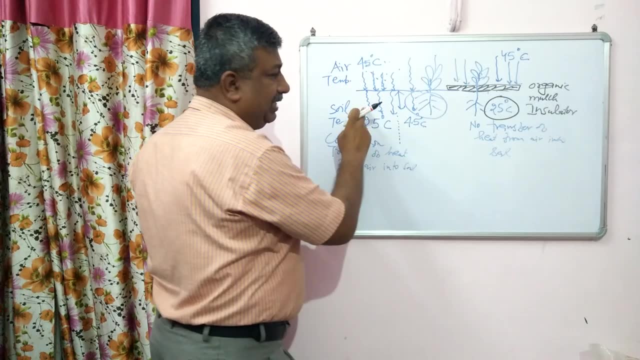 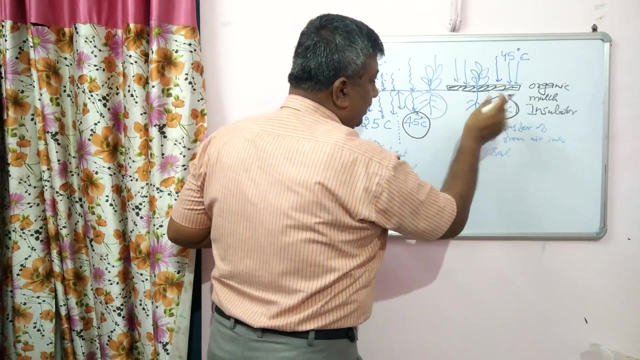 it is 45 degree centigrade. Temperature is increasing and it is increased, but it is not transferred into the soil as in case. so temperature remain 25 degree centigrade. Here temperature is 45 degree centigrade and now temperature is in optimum. we can say: 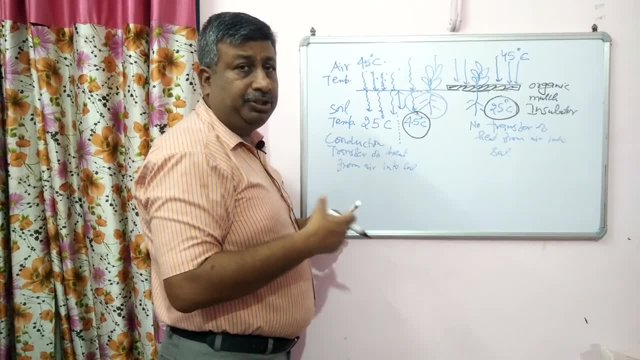 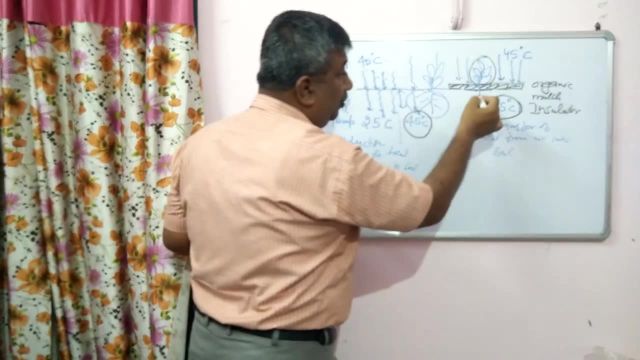 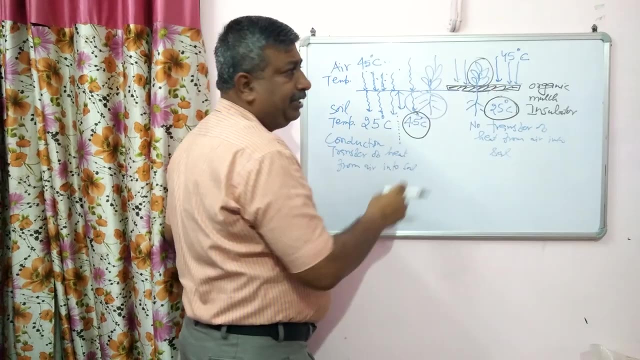 rain, so roots absorb properly moisture, nutrient and translocation. no doubt here plant is suffering from the heat. High temperature is there, But root zone, which is responsible for absorption of nutrient, face or experience the low temperature as compared to air temperature. so root activities are maintained. 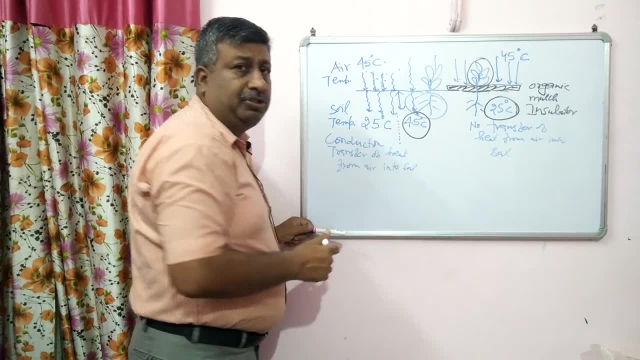 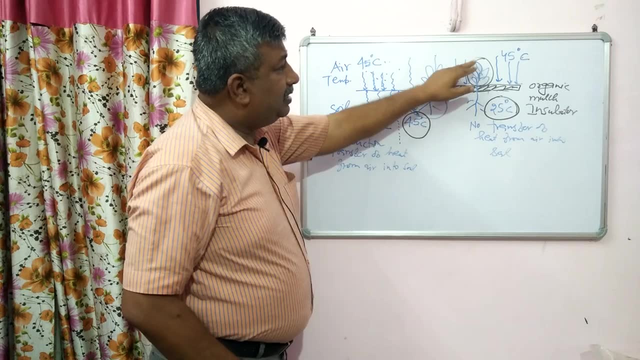 So there is no severe loss, while in case of this, where organic mulch is not used, there is severe loss in the growth and the yield. So here, in this case, the plant's leaves, in that the air temperature is high, but in the roots the temperature is not high and it is maintained in this zone. 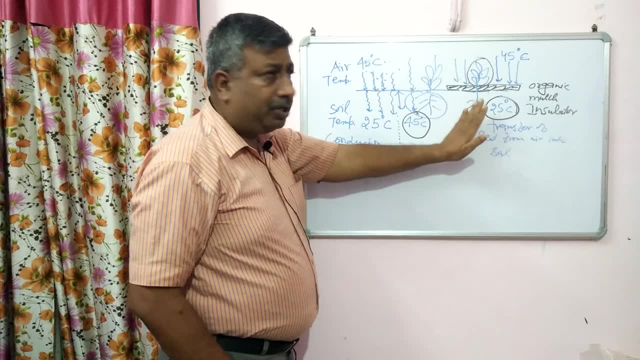 So in this case the plant's leaves, in that the air temperature is high, but in the roots the temperature is not high And in this zone it is maintained. So here there is proper nutrient absorption translocation and from here the water absorption is happening. 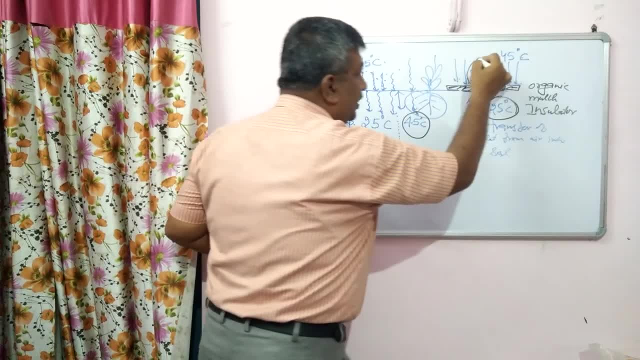 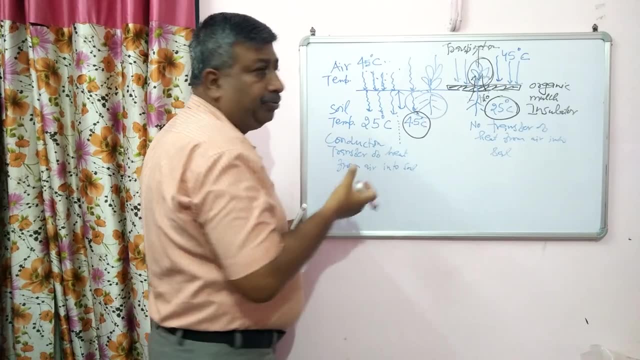 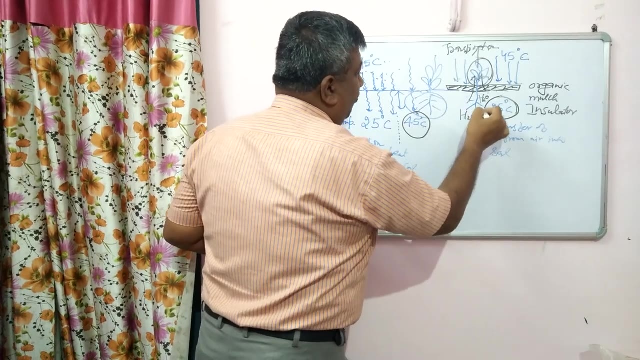 Now this water is translocated to the upper part. Now this water is transpired, There is a transpiration. So now, here, transpiration is maintained because roots are able to absorb the moisture, because temperature is in favorable zone or range. So water absorption is there. it is translocated to upper part. transpiration is there, so that's. 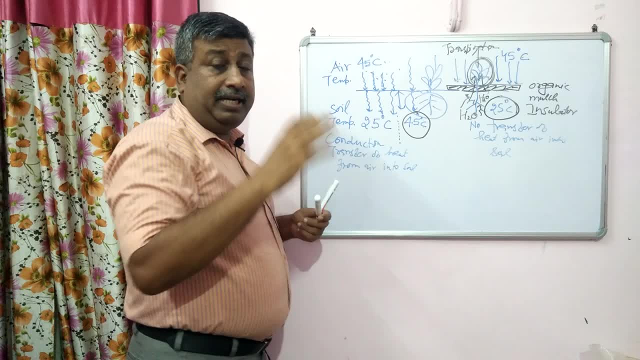 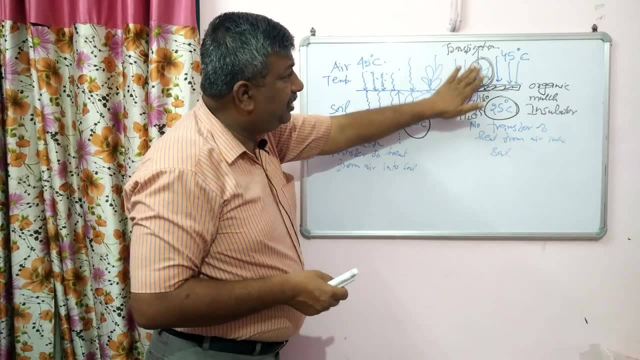 why a cooling effect is maintained, So high air temperature is minimized, reduced. So here roots are absorbing water, plants are translocated and there will be transpiration there, so the cooling effect will be maintained and the adverse effect of high temperature will be minimized. 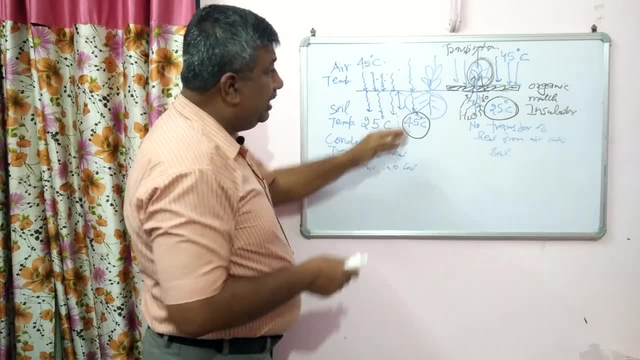 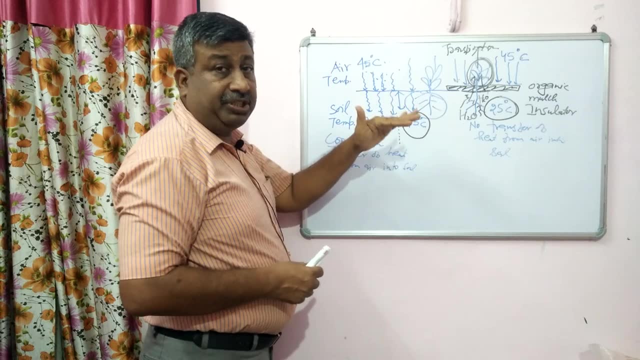 But in case here there is no water absorption so this plant face root, face high temperature, shoot face high temperature. so there is severe reduction in growth and yield. But if we use the organic mulch then we can reduce the adverse impact of high temperature. 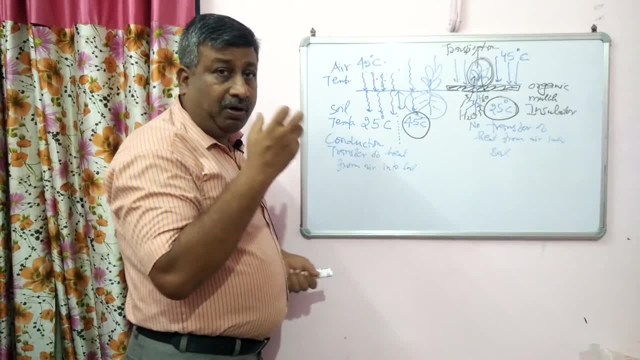 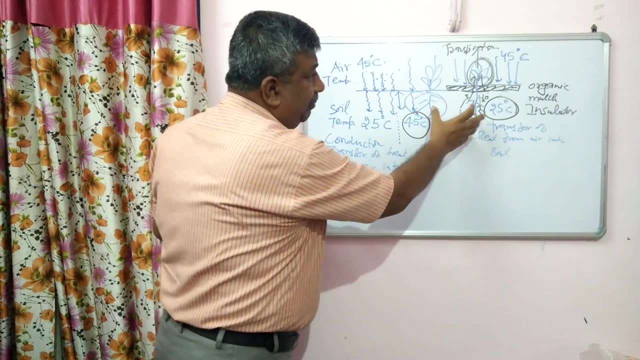 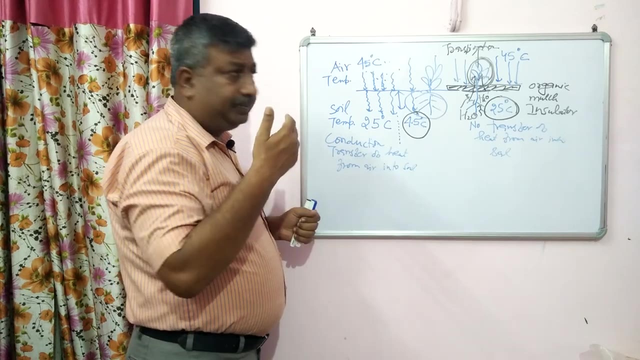 So this is the root structure. we are using temperature. so this is the effect of temporary or effect of organic mulch to reduce the or to maintain the low soil temperature as compared to air temperature. so this is the beneficial role. so in summer season, other if this. 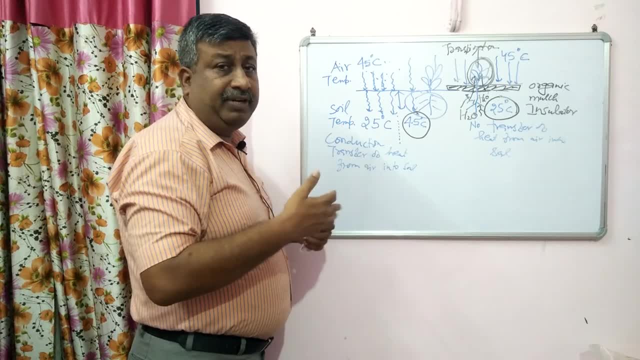 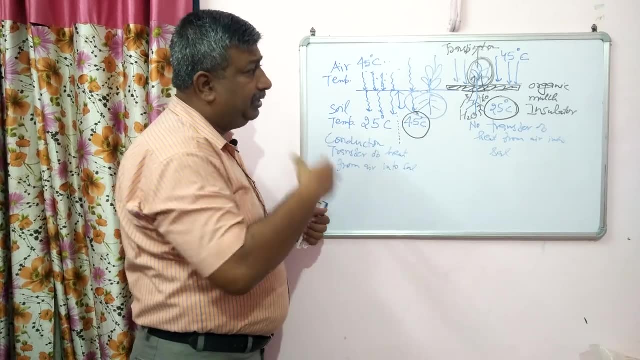 organic mulch are applied into the crop, we can get very good yield to other summer season quick crop grow kar raha hai or maha soil from organic mulch ko use karein, toh bahut achcha impact hame nazar aiga ki iss se soil temperature. kaise? 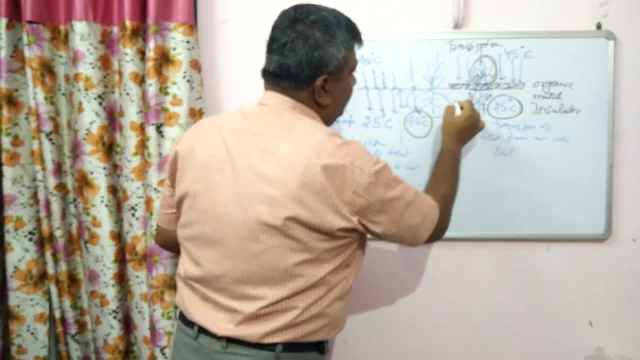 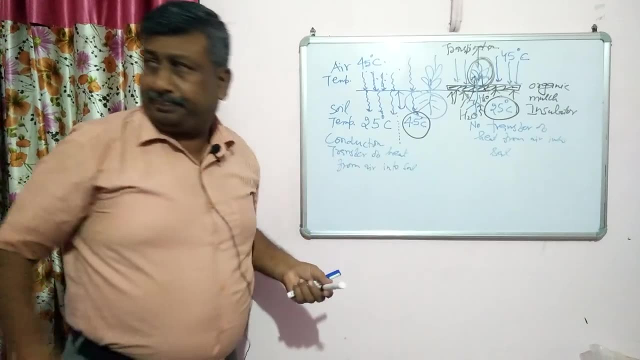 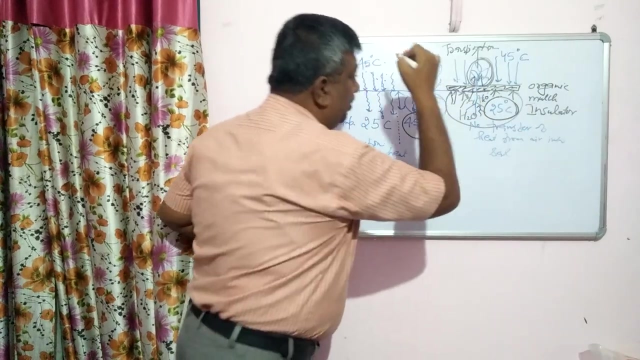 regulate hota hai. uska additional advantage: dosa kya hai if there is evaporation of water. so now organic mulch is there, so it restricts the evaporation. restricts the evaporation, so water is also maintained. so regulation of moisture as well as temperature. so this is a beneficial role, so it prevent. the moisture loss and regulate this soil temperature. So this is the reason that organic mulch play a very important role in increasing growth and yield in summer season. Now what happens if this organic mulch are used in winter season? If we are using organic mulch in winter season, then what is its impact? Now this is the soil surface and this is the plant and temperature is 25 degree centigrade And in winter season- now season is changed- winter season temperature is suppose 10 degree centigrade or 5 degree centigrade. Now there is a high temperature in root and in winter. 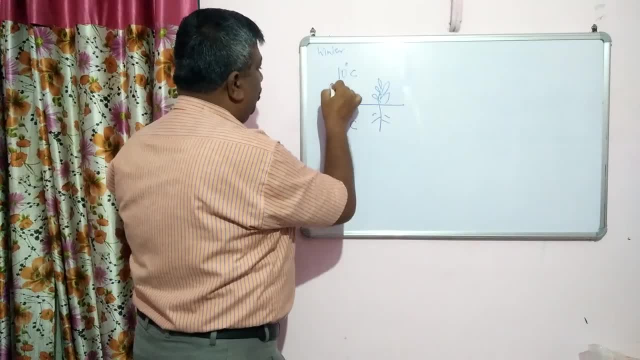 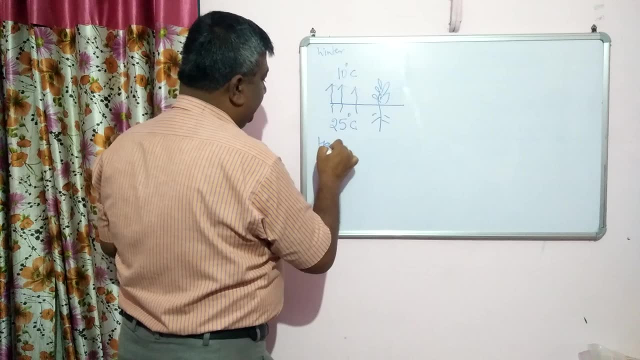 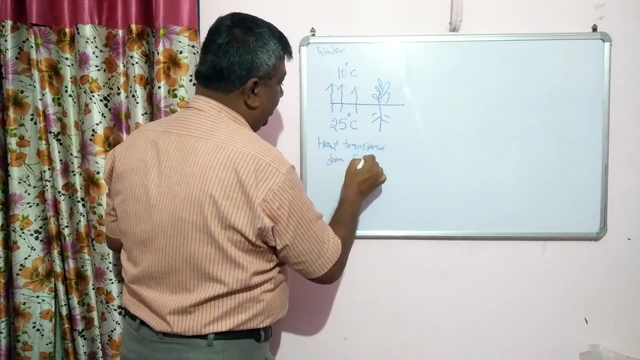 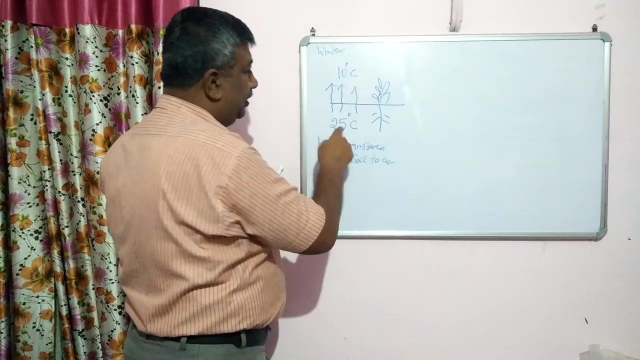 season, air temperature is low as compared to soil temperature, So there is a loss of heat. So now the heat is transferred. heat is transferred from soil, heat transferred from soil to air. Now, because of this continuous loss of from this soil to air, temperature is equilibrium. 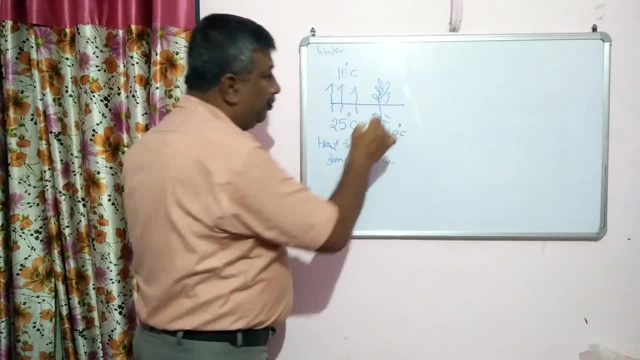 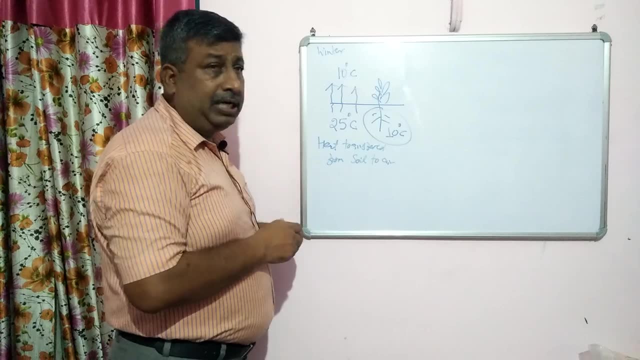 with the air temperature and it is 10 degree centigrade Now. root phase low temperature and because of this low temperature, poor absorption of nutrient and the moisture and the growth is affected. So shoot, growth is affected because of low air temperature. Now, roots are adversely affected because of low soil temperature, because there is a continuous loss of heat from soil to air. and in summer season what was happening? in summer season There was a heat transfer from air to into the soil, But here soil temperature is high. 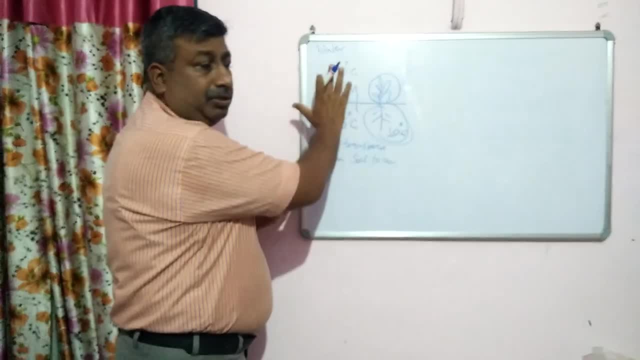 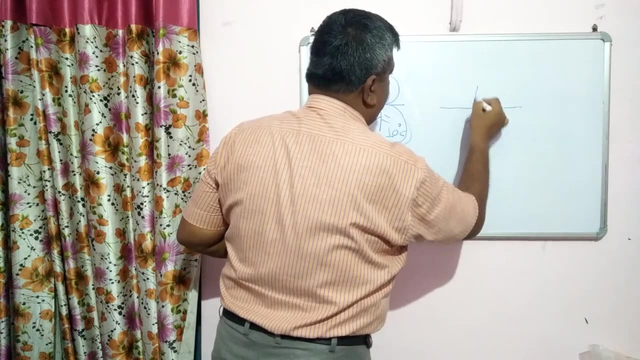 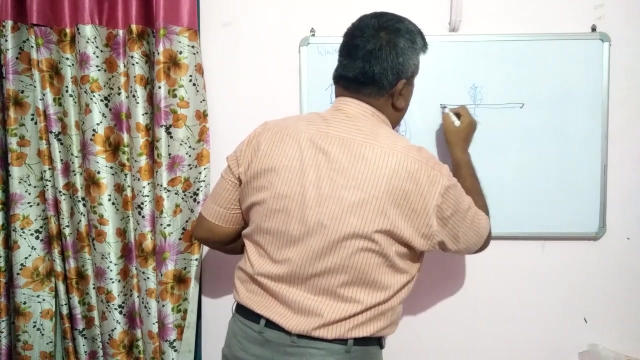 and air temperature is low- Suppose it is 5 degree centigrade- then further loss of heat. Now suppose we are using the organic mulch and this is the plant and temperature. and we are using the organic mulch like that: we are spreading the crop residue or straw or